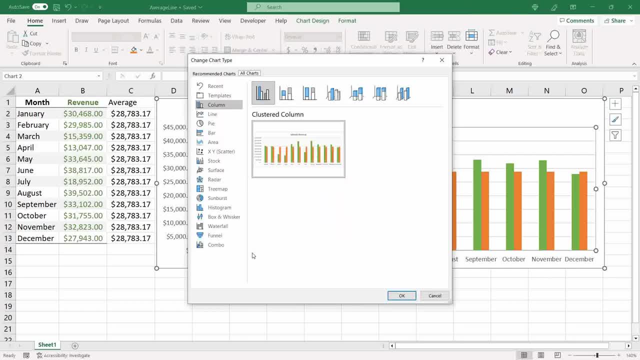 and click on change chart type. This last option, called combo, will allow you to change the chart type for each series. In our case, Excel is already recommending the line chart for the average function, The average series. if it was not here, you can select the chart that you, the chart type that you. 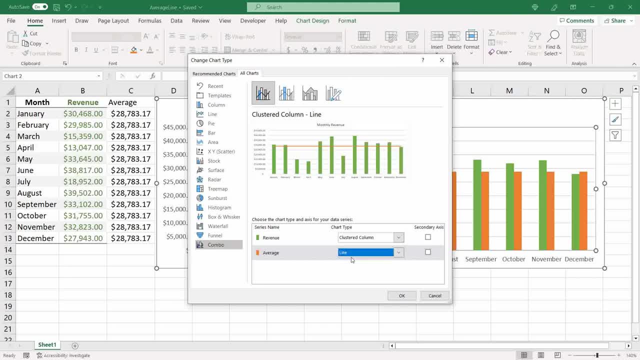 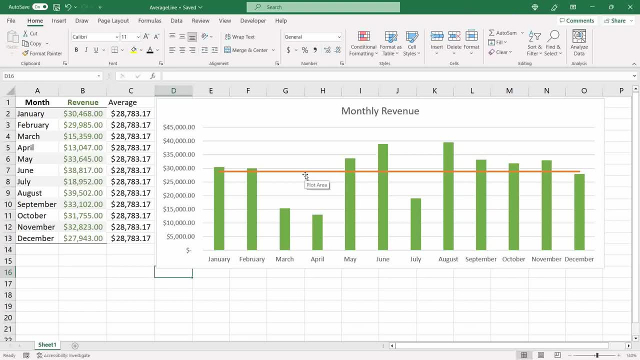 want in this arrow, just besides the, the name, It's line already. I'll click okay. Now we want to change the line type for a more dash to one. Personally, I prefer- I don't like- solid lines for the average value. so right click over the series and select format: data series and. here in this box, I can see that I have two lines. I can also change the line type for the average. I have the same thing here. I can add an additional line type and I don't need to change the line type for the average as well. so you can see my data Right. So I have the same thing here. I can add: 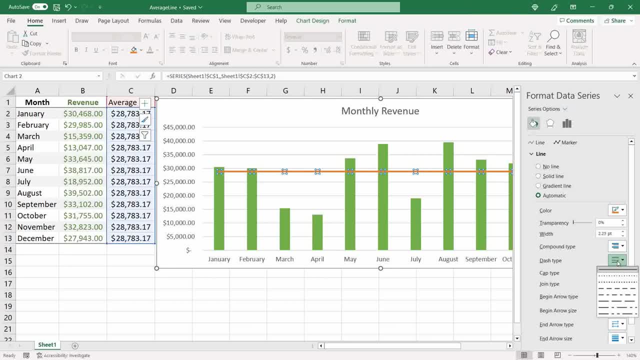 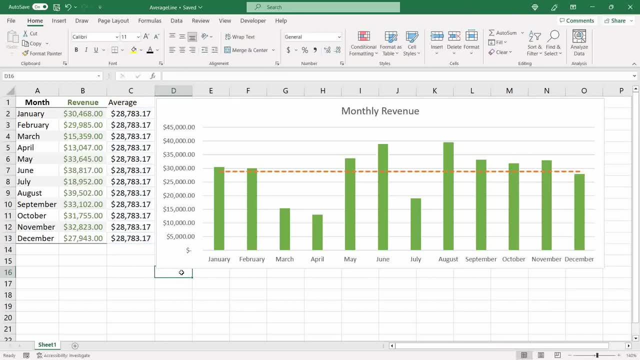 a new line to this one. I can also change the line type to if I want to change the line that I want in this clip. If you don't see the line, there's another box called fill line. under the dash type, I'll select the third option, called square dot. Perfect. Now we want to add the label for the. 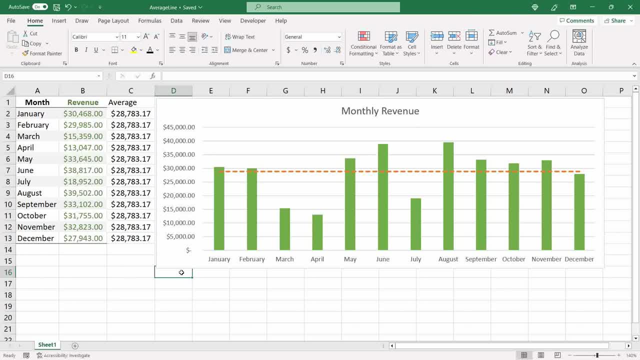 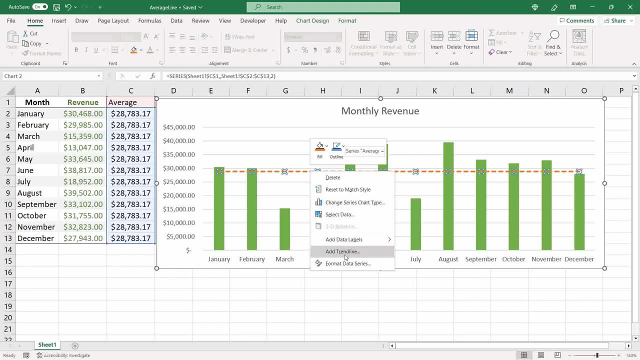 annual average. Let's say we think it is important to know the average value for the year, but if you right click over the series and select add data label, Excel will add the data label for each month and we don't want that to solve this problem. after you select the series, the average series- 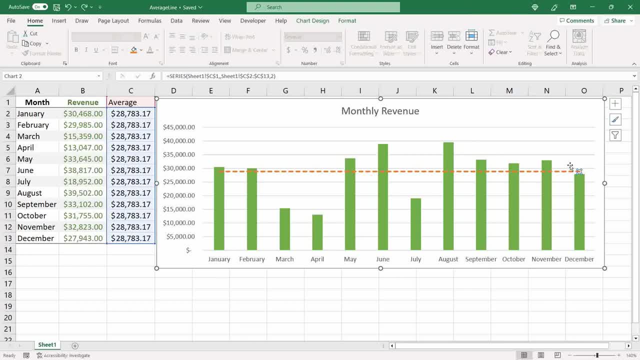 select again. click again on the dot that you want the value to be added. i like to add it in the last one and then notice that now we have only this dot select, and then right click over it and select add data label. however, our label is in the middle of the line. it's in the top of the bar. 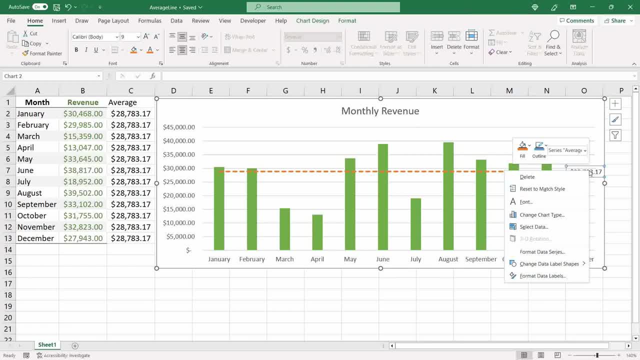 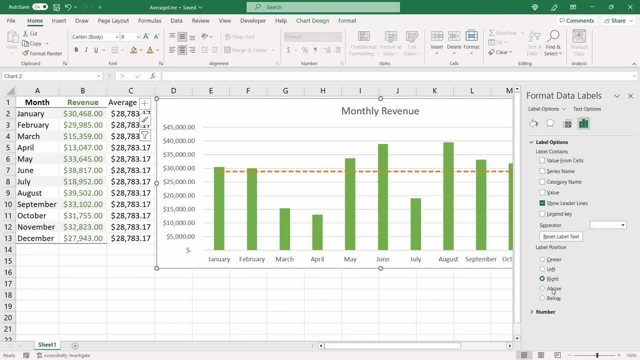 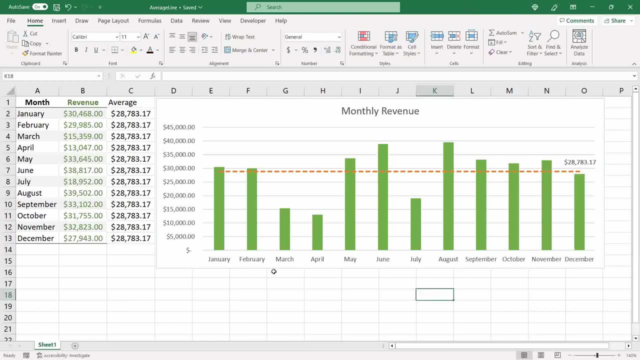 it's not very clear to change the position, right click over the label and select format data labels and switch the label position from right to above under this menu called the label positions close. however, personally i like to make an extra space in the chart, if it is possible, just for the